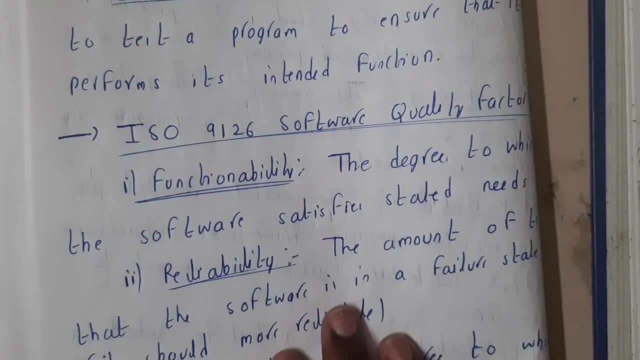 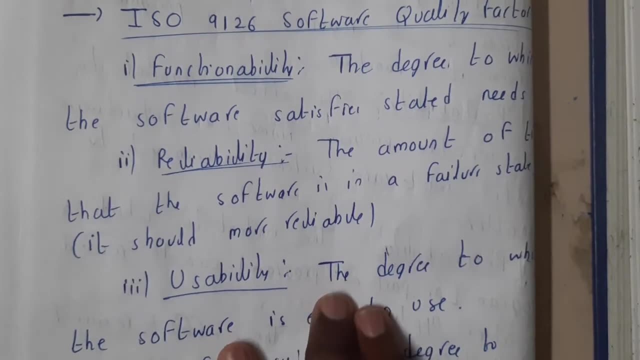 we will be making these things guys, So we will be writing the functions and everything Similarly. reliability. So whenever there is a failure in the system, the entire system should not go down. and even though, if there is a technical issue and if everything goes, 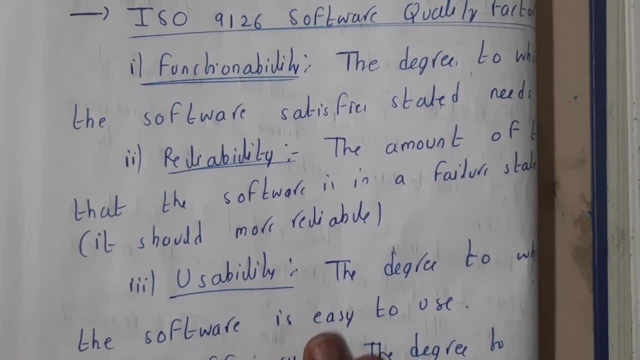 down. the operations that are need to be done should be really faster, guys. So it should be done in a way that it should be done in a way that it should be done in a way that they should not waste the time of the user. So it is valuable. So the amount. 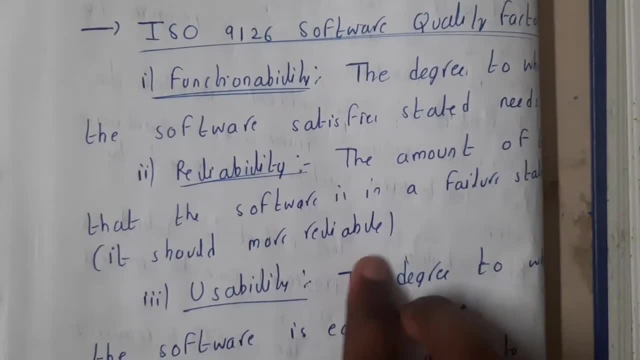 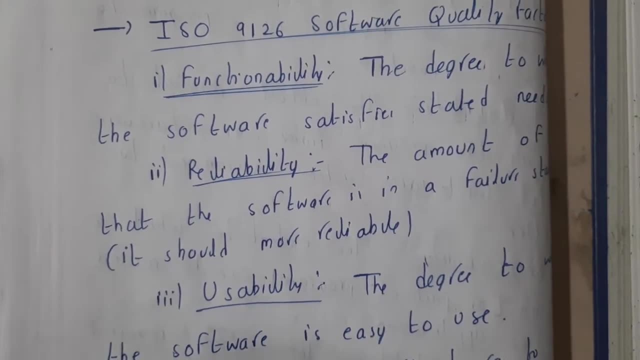 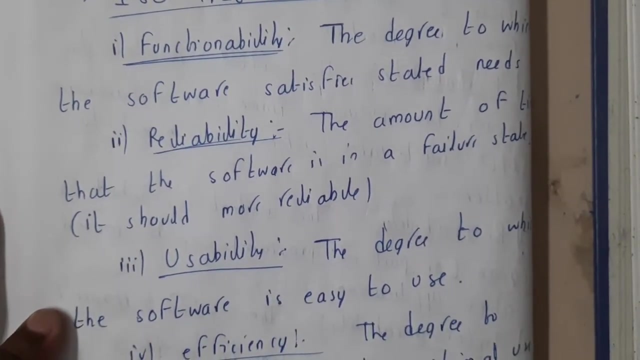 of time that is required for a software to recover from the failure is nothing but reliable guys. So if it is recovering in a faster way, we can say that the device or the product or the software is more reliable. Usability: The degree at which the software is easy to. 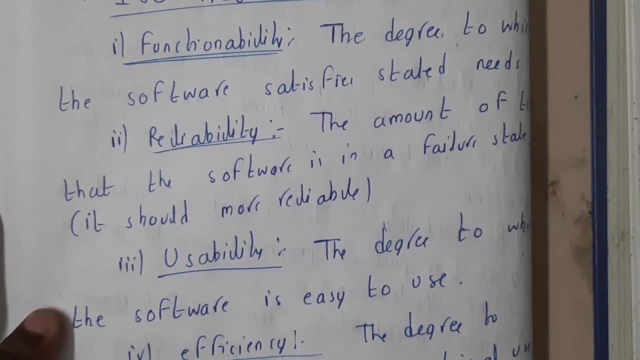 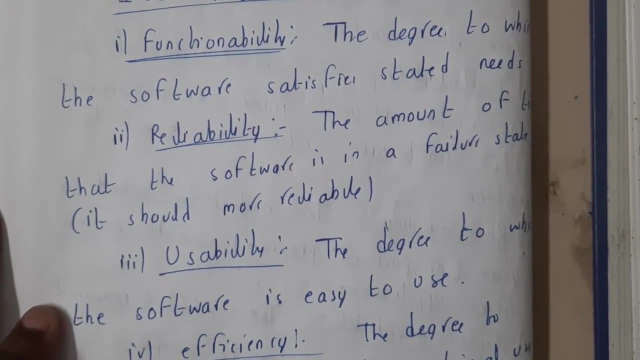 use. So basically, most of the users are non-technical guys. They will not be having technical knowledge Like a programmer, but they can operate and they can use multiple applications. So that is the major advantage. So even nowadays the kids are opening YouTube and they can. 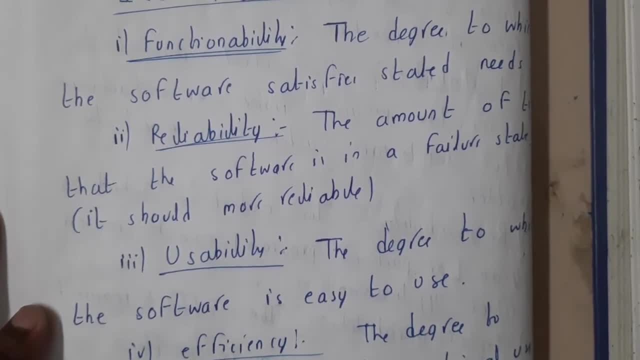 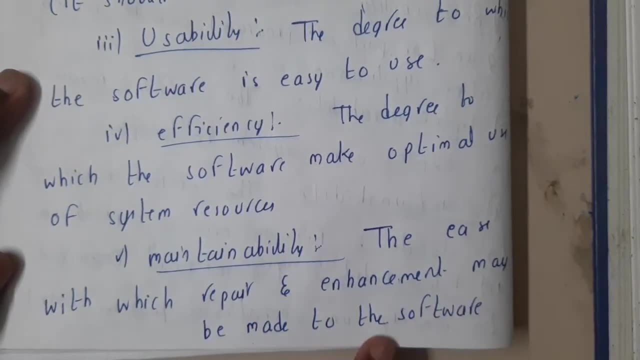 play their rhymes or any kind of YouTube videos, Right? Yes, Similarly, maintenance, So the ease with which a repair and enhancement may be made to be the software. So maintenance is nothing, but you will be frequently checking for any kind of issues and, if you find any, 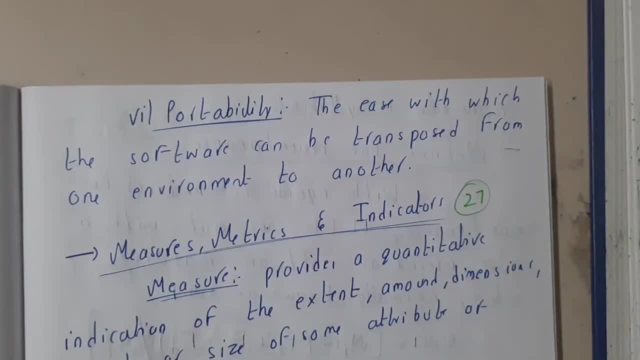 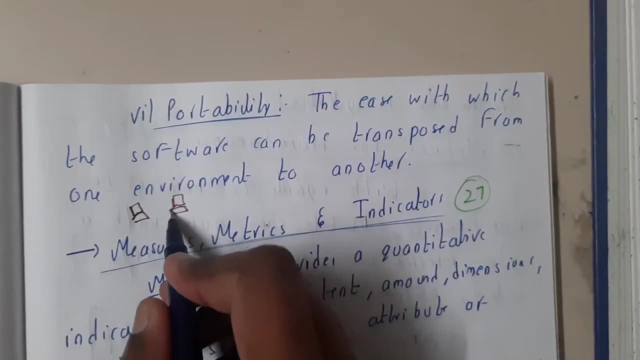 issues, you will be resolving them. Portability: So we discussed about portability previously also. So assume that I wrote a code on my Windows system and I want to transfer it to my friend who is having a Mac system. So if I transfer the file, like in C or C++, the 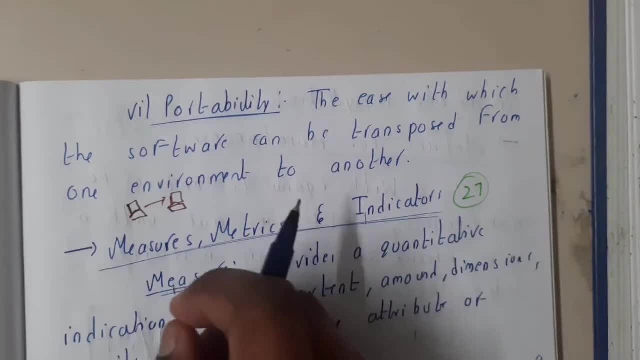 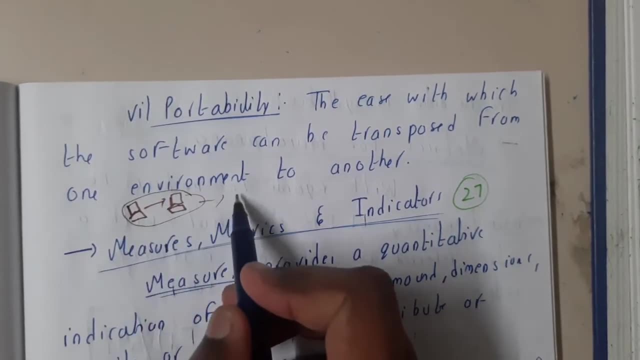 files cannot be run directly on my friend's system. guys, If I send only C or C++ files, That is nothing but c and c++. Basically, if you send the same program of a Java from one system to another system or Python from one system to another system, you will not. 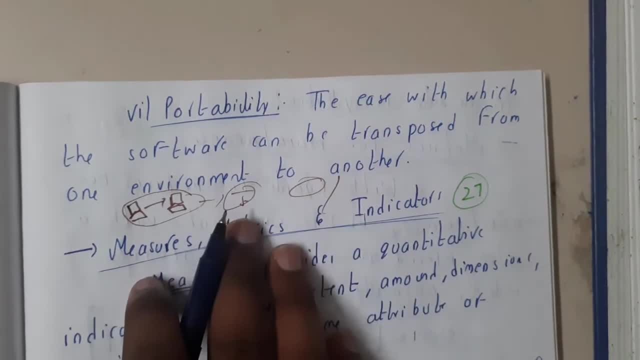 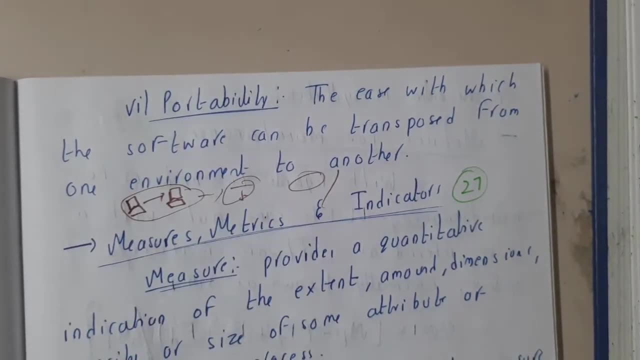 have this problem, guys, Because both the languages are portable, Which means the ease with which the software can be transported from one machine or one environment to another. Okay, So I hope everyone got some basic idea. So in the next lecture we will be going through one of the three of the most important words. That is nothing.